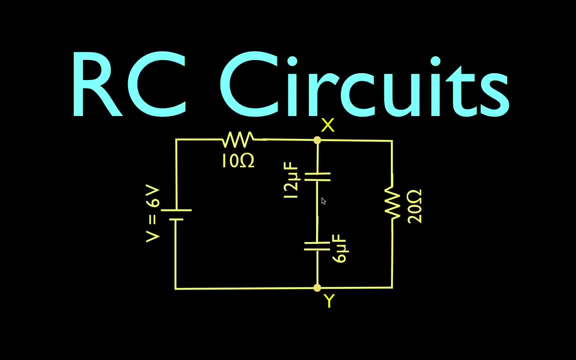 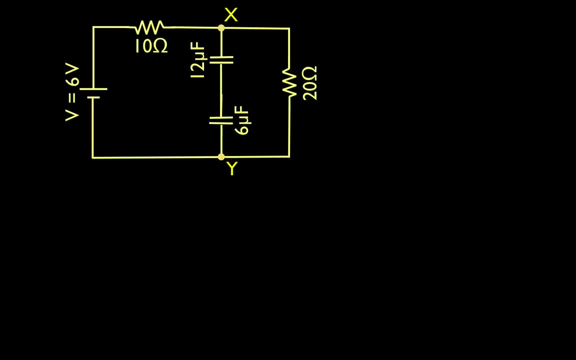 6 and a 12 ohm- excuse me, 6- and a 12 microfarad capacitors. So this is our RC circuit. You will notice also that we have a 6 volt power supply And this is the circuit we're going to use. 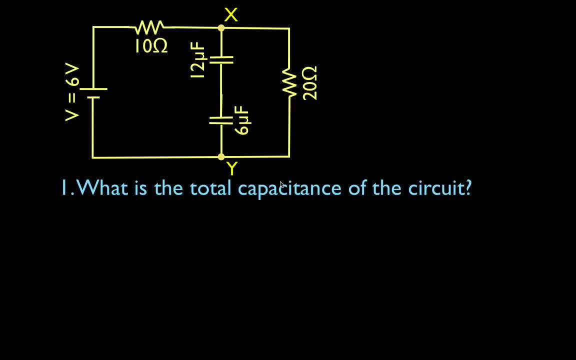 And these are the questions that we are going to try to answer for this circuit. What is the total capacitance of this circuit? What is the current through the 10 ohm resistor? What is the potential difference from point X to point Y? What is the charge that is stored on the 6 microfarad capacitor? 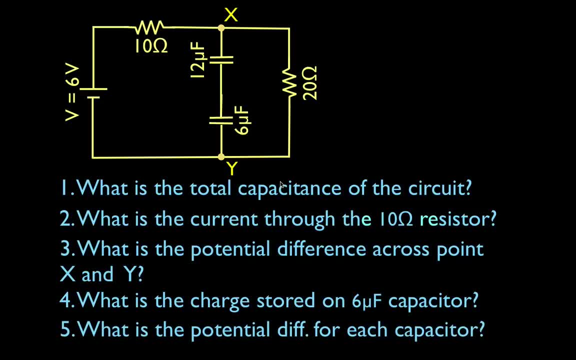 And what is the potential difference between the 6 and a 12 microfarad capacitors For each capacitor. Now, we're going to do this from this perspective that the circuit has been closed and running for a long time. If we had a switch, we'd close the switch. The switch is. 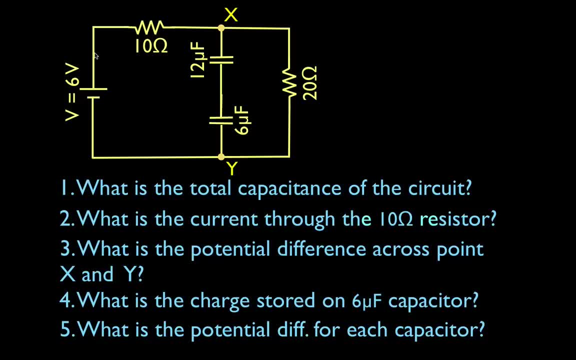 closed. We are at time equals infinity or a long time. Now what does that mean? when we say that This is what it means, It means the current has been running, the switch, the circuit has been turned on And basically what it means is that the 2 and a 12 microfarad capacitors are running. 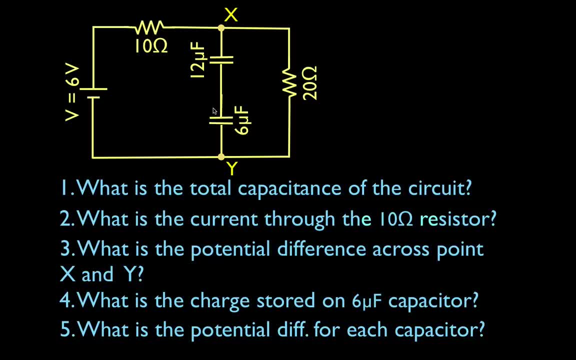 through this outer branch of the circuit. The circuit is fully charged. And here's the difference: The current continues to run through one of the capacitors of the circuit, So the current continues to run through and the two capacitors are fully charged. Okay, They're fully. 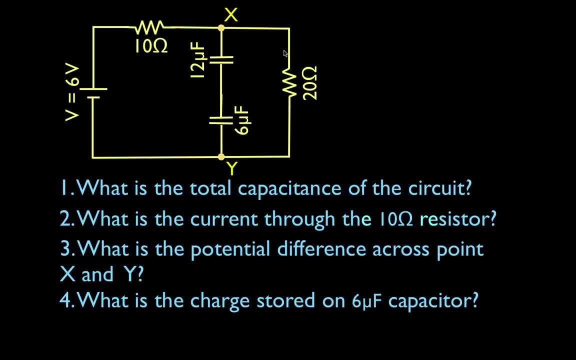 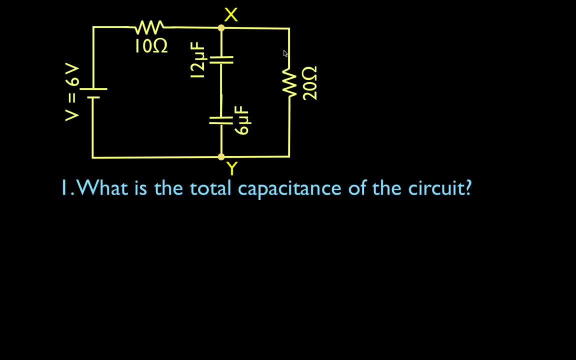 charged and then the current continues to run through this outer branch of the circuit. So two things: the capacitors are charged and the current is running through those two capacitors. Okay, let's get on with this. We want to try to finish this in 10 minutes or less. What is the total? 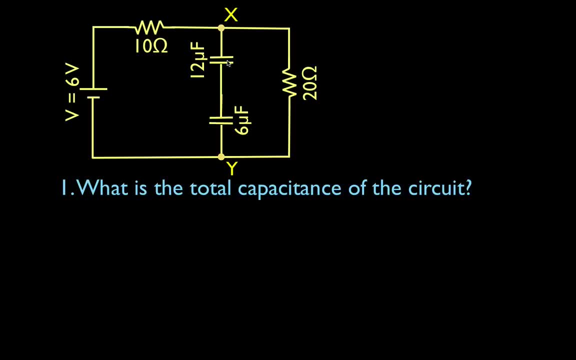 need to find the total capacitance of those two capacitors. those two capacitors are in series, so we're going to use our series equation for capacitors, which is one over the total capacitance is equal to one over the capacitance of the six microfarad capacitor, plus one over the capacitance. 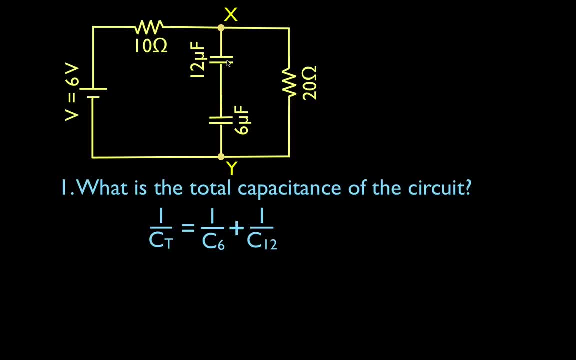 of the 12 microfarad capacitor. all right with, these are not in parallel. if they were in parallel we could simply add them up. six and twelve would be 18, but we're in when they're in series we have to use the one over equation. so we have that the total capacitance is one over six plus one over 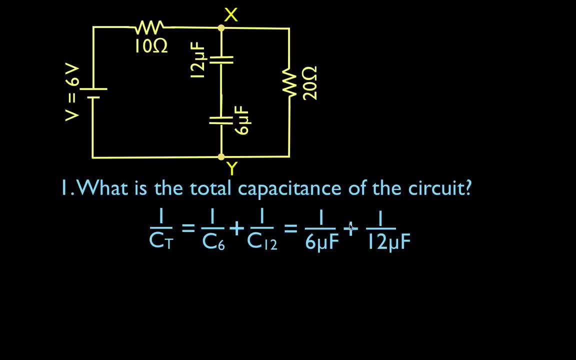 twelve. i just in my calculator put one divided by six plus one divided by twelve and i get that one over the total capacitance is equal to 0.25 microfarads. now it is important to remember that this is not the total capacitance. this is one over the total capacitance to get the total. 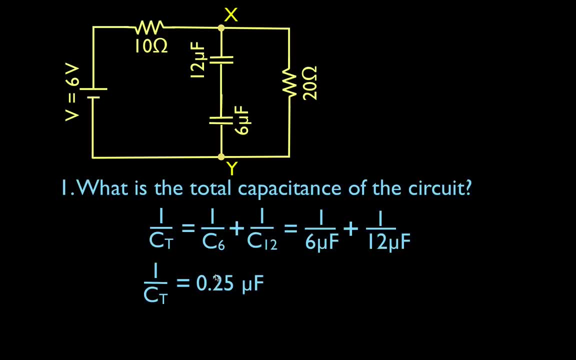 capacitance. i must now take the reciprocal of this side and the reciprocal of this side, and if i do that, i get the total capacitance of the six microfarad capacitor plus one over. the total capacitance is equal to one over 0.25 microfarads, which means that the total capacitance, the 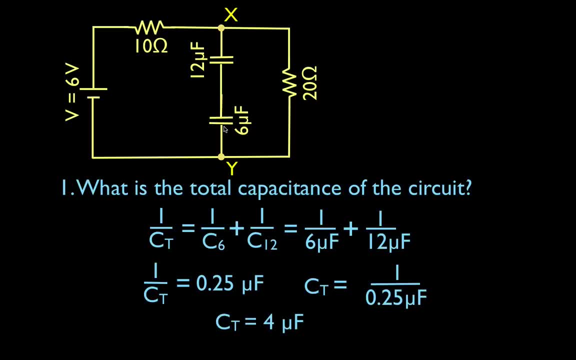 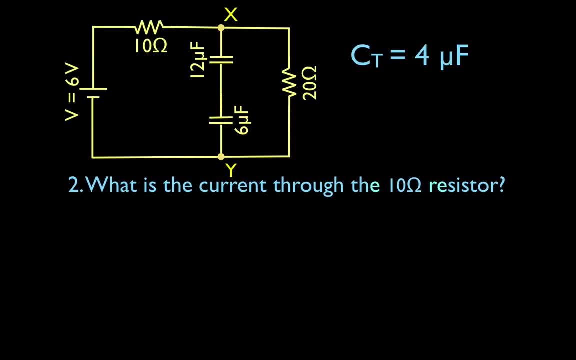 equivalent capacitance of these two capacitors in series is four microfarads. so that is the total capacitance of that circuit. okay, number one. number two: what is the current through the 10 ohm resistor? now, we said the current is running. we're in steady state, the capacitors are charged, the 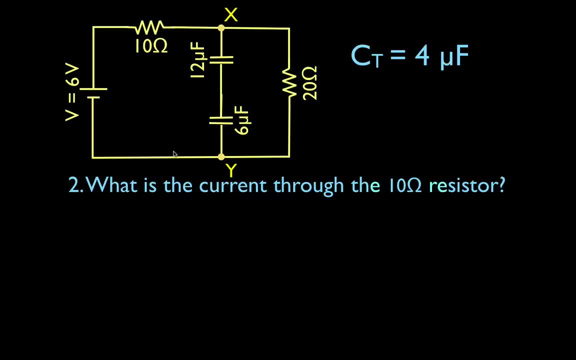 current is running through this outer branch. there are no capacitors, there's nothing blocking the current in this outer branch. so now we have a 10 and a 20 that are in series. the current through each of these is going to be the same. that's the current rule for resistors in series, the current 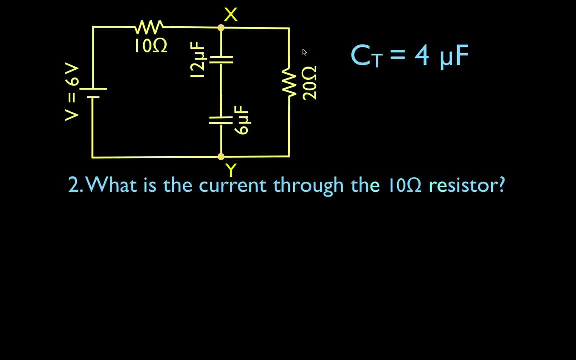 is going to be the same. so if we can figure out the current through the 10, then we also know the current through the 20, and if we can use our v equals ir ohm's law to do that, okay, we know the voltage. now we're. 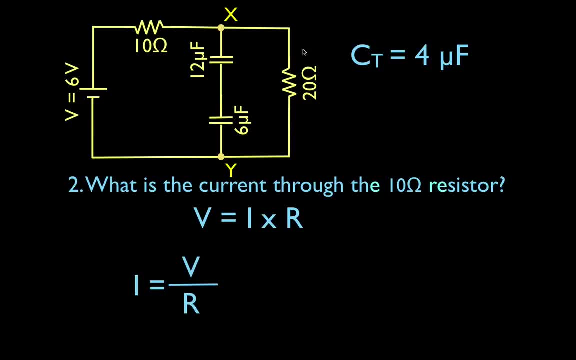 solving for the current. the current is the velocity divided by the velocity, the voltage divided by the resistance. okay, the total voltage- there's only one voltage- is six volts. now we have to use the total resistance and because these two resistors are in series, we just add them up in: 10 and 20 is. 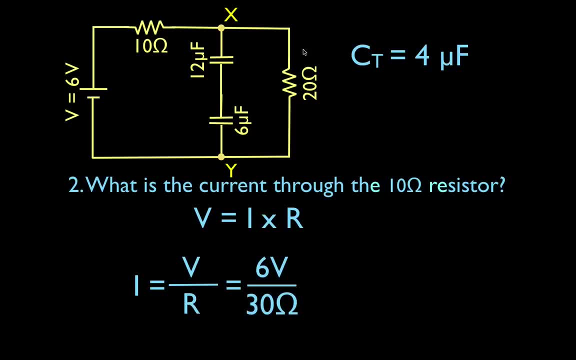 30. okay, so now we're kind of finding the total current through the circuit, but there's only one branch, so that's going to be the same in both, which is 0.25 amps. so now we know the current through this resistor and this resistor and any point in this. 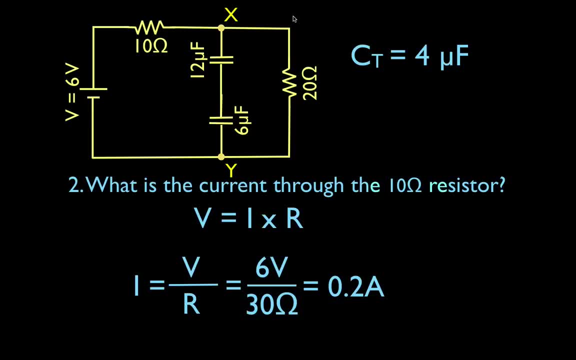 outer branch is 0.25 amps. okay, so that's how you find the current through the 10 ohm resistor. now we're going to find the potential difference across point x and y. so if we measure the potential difference from this point to this point, what will it be now? this is another thing you have. 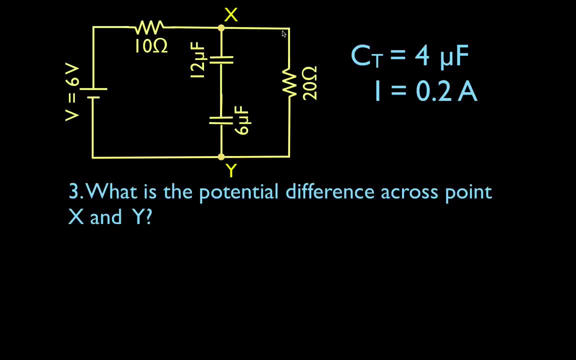 to remember these two branches: this branch and this branch are in parallel. the voltage across parallel branches in a circuit is the same. so if we can find the voltage across this branch, then we'll know the voltage across this branch, because it's the same thing. okay, basically, anywhere you measure the current, the 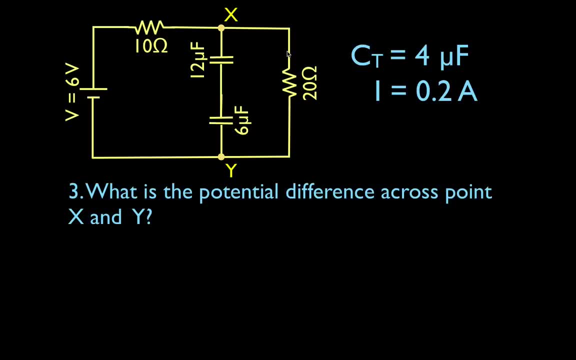 voltage along here. as compared to along here, it's going to be the same, so we can get pretty easily the voltage across the 20 because we can use our ohms law. okay, now the question is from x to y. so i put down here voltage x to y. but really, 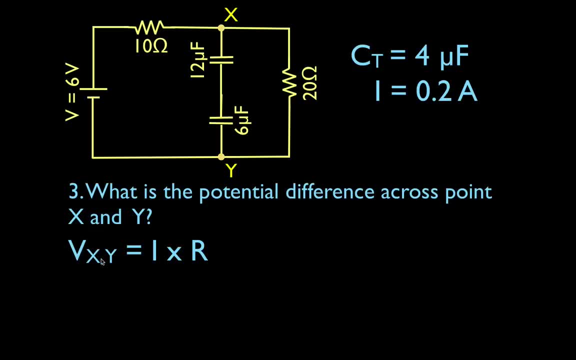 the way i think about it, what we're really calculating is the voltage across the 20 ohm resistor, because we know the current, we know it's 0.2 amps, we know the resistance: it's 20 ohms. so that means that the voltage from x to y, the voltage across the 20 ohm resistor, is 4 volts. well, that's. 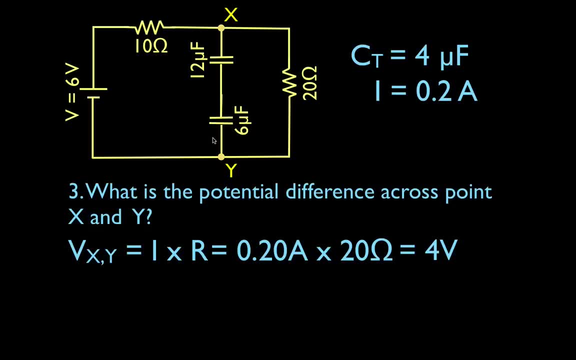 in parallel to these two, the branch that contains these two capacitors. so that's going to be the same. now we could, and maybe we should, just to check. let's find the voltage drop across the 10 ohm resistor, because we know you are used 4 volts on the 20. then this should really equal 2, so the 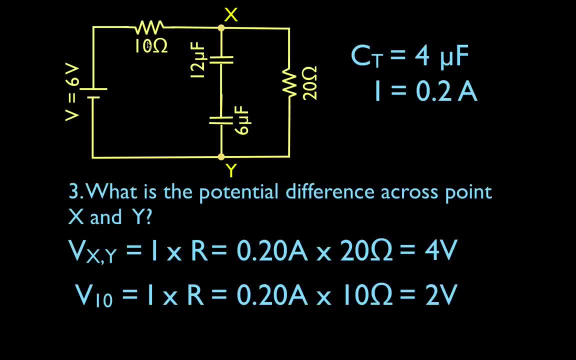 voltage across the 10 is its current, which is the same times its resistance, which is 10 and that's 2, so these two have now added up to 6 and that's 6. you know, when you go around a loop, the voltage has to be the voltage drops and the voltage gains have to be equal to each other. okay, 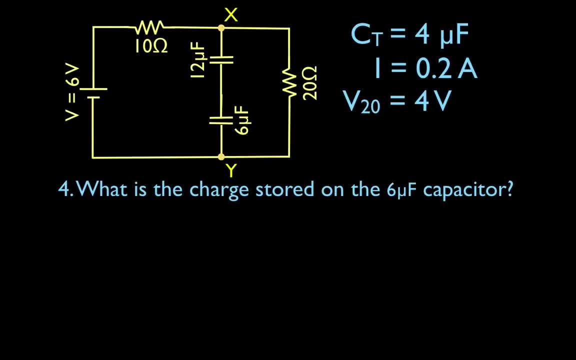 and we got that. now, number three: what is the charge stored on the six microfarad capacitor? okay, now this is something else you need to remember. we have two capacitors in series. all right, we figured out the total charge. excuse me, we figured out the total charge. the total capacitance is four. all right, microfarads. now you need to remember. 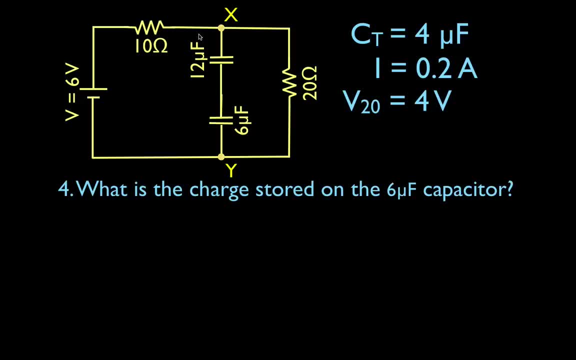 for capacitors in series that the total charge and the charge on each capacitor is the same. so the charge on this capacitor, okay, and the charge on this capacitor is going to be the same and they're going to equal the total charge. so we're going to use: q equals c times v. 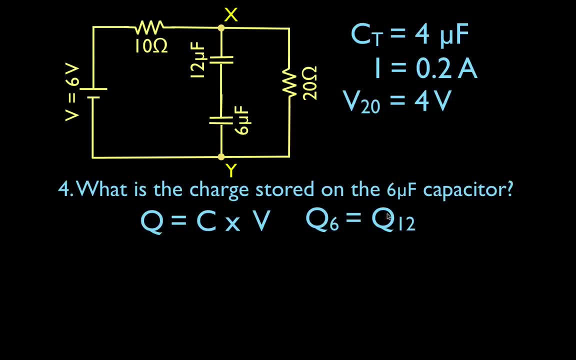 and we know that the charge on the 6 and the charge on the 12 are the same and they also equal the total charge. that's the rule for capacitors in series. well, we can figure out the charge on the 6 and the 12 together because they have the same charge, not equal to the total. 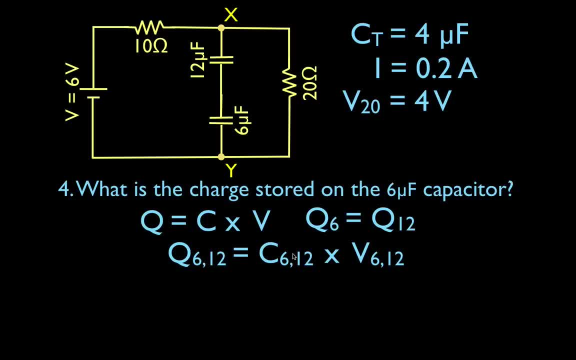 so what do they do? is equal to the capacitance of the 6 and the 12 times the voltage across the six and the 12, across both of them, across that whole branch. so we know that the equivalent capacitance, the total capacitance of those two, is four microfarads. we know the voltage across each of those, across both of them. excuse me, cross both of them. 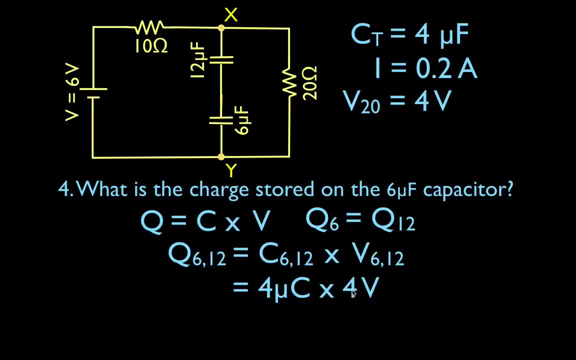 is 4 volts. Therefore, we just multiply those two together, the total charge, the total capacitance, the total voltage, and you get that the charge stored on the 6 and the charge stored on the 12, and the total amount of charge stored is 16 microcoulombs. okay, That's, I would say. 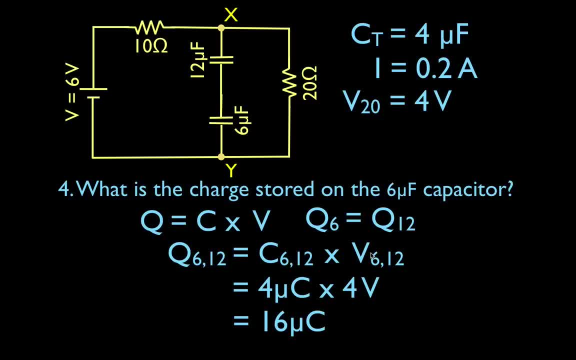 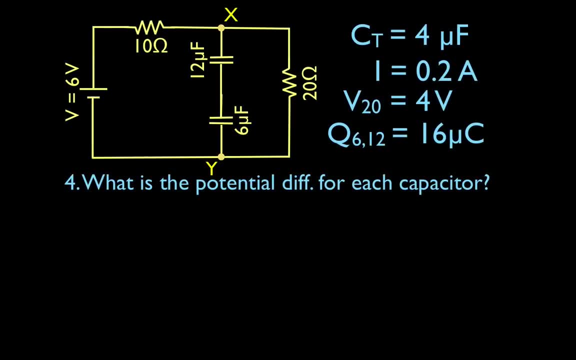 that's the trickiest part of this. Remember the charge rule for series capacitors? all right, All right, the last one. Now we can get the potential difference across each capacitor. Well, once again we're going to go with Q equals C times V. naught, V equals I times R, because we